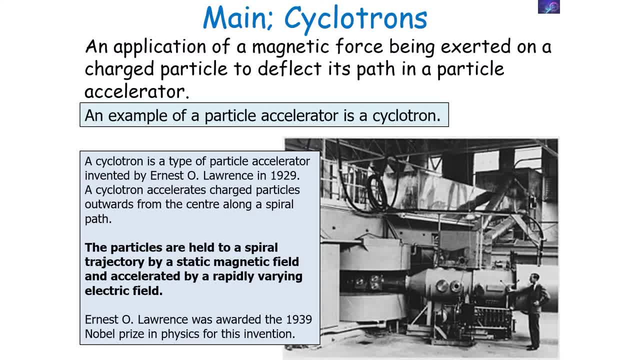 Now, an application of a magnetic force being exerted on a charged particle to deflect its path is a particle accelerator. Now, an example of a particle accelerator is a cyclotron. Now, a cyclotron is a type of particle accelerator invented by Ernest Lawrence in 1929.. 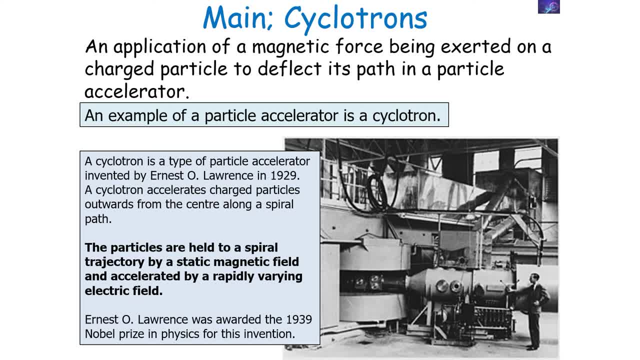 So a cyclotron. cyclotron accelerates charged particles outwards from the centre along a spiral path. Now the particles are held to a spiral trajectory by a magnetic field and are accelerated by a varying electrical field. Now Lawrence was actually awarded the Nobel Prize in 1939 for this invention. So the 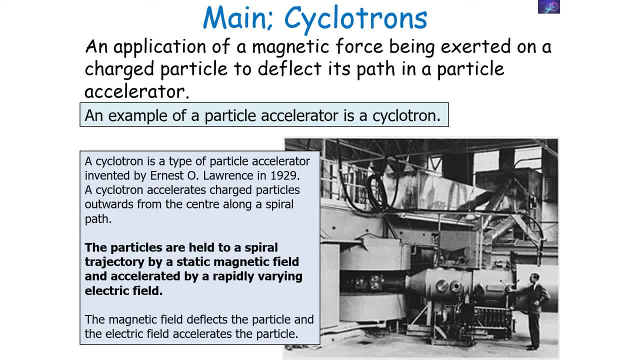 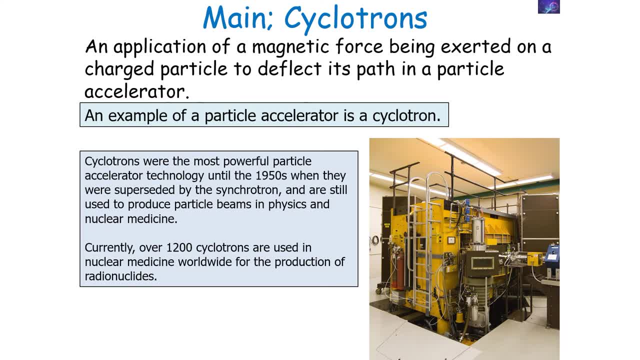 magnetic field deflects the particle, and the electrical field accelerates the particle by changing its speed. So cyclotrons were the most powerful particle accelerator until about the 1950s, when they were superseded by the synchrotron, but are still used to produce particle beams in 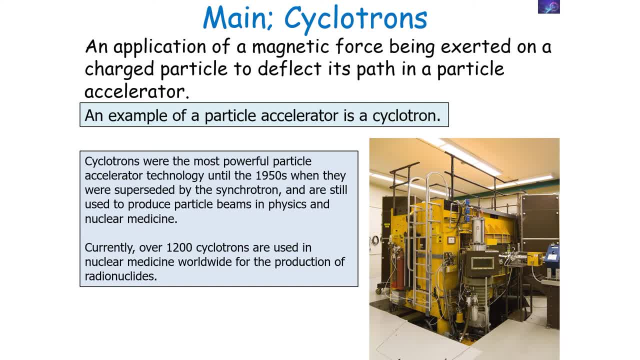 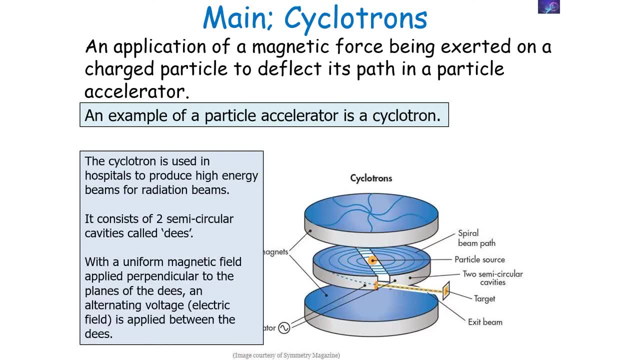 physics and nuclear medicine, and currently there are over 1,200 cyclotrons used in nuclear medicine worldwide for the production of radionucleotides. So a cyclotron is used in hospitals to produce high energy beams for radiation and it consists of two circular cavities or discs, which we call. 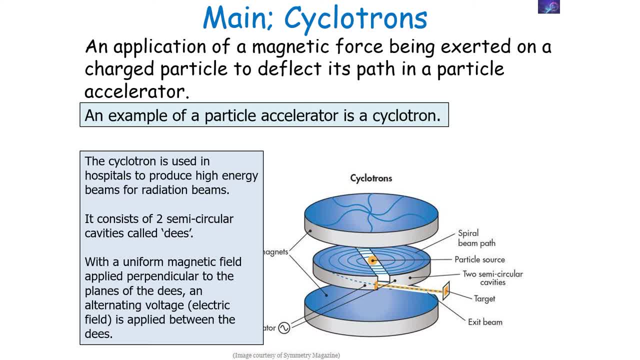 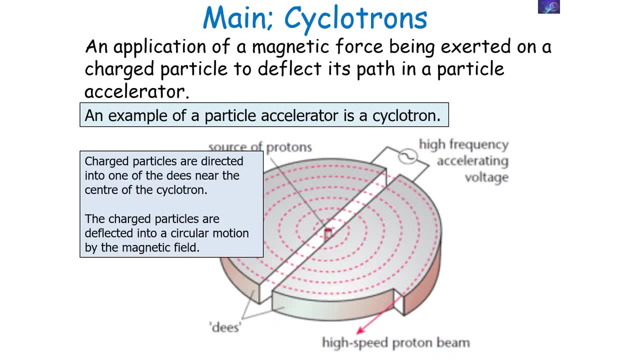 D's. Now, with a uniform magnetic field applied perpendicular to the planes of the D's, an alternating voltage at potential difference is applied between the D's, So charged particles are directed into one of the D's near the centre of the cyclotron. The charged particles are deflected into a circular motion. 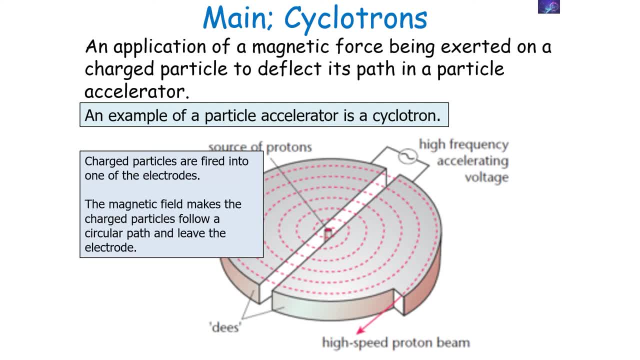 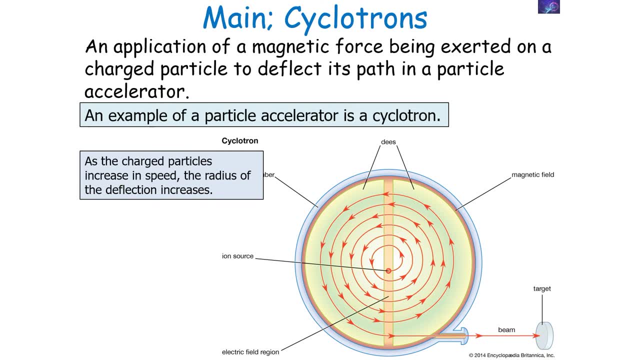 by the magnetic field. So the charged particles are fired into one of the electrodes and the magnetic field makes the charged particles follow a circular path and leave the electrode. So as the charged particles increase in speed, the radius of the deflection increases. We know this from the 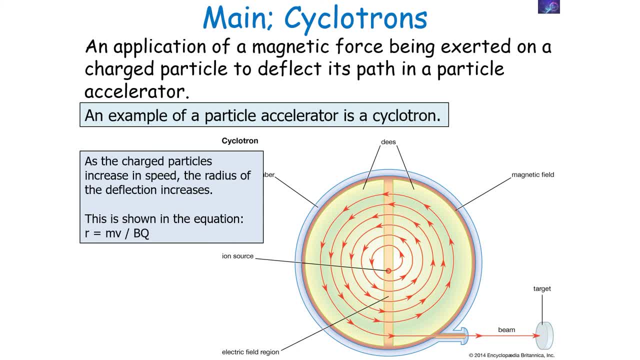 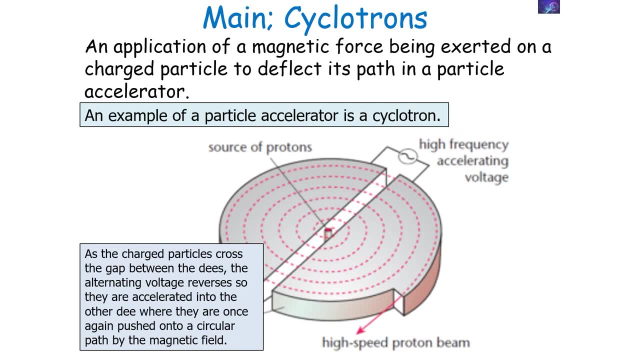 equation: r equals mv over bq. increasing R is increasing, so the particles follow a spiral path where the radius is increasing. Now, as the charged particles cross the gap between the D's, the alternating voltage or potential difference reverses, so they are accelerated into the other D where they 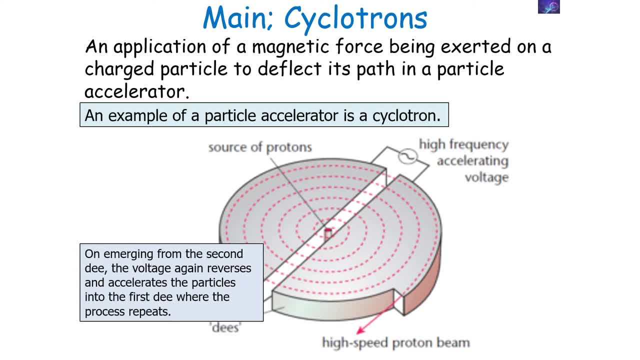 are once again pushed onto a circular path by the magnetic field. Once emerging from that second D, the voltage again reverses and accelerates the particles into the first D, where the process repeats. Now, if the potential difference was not alternating, what this would cause? we would cause the 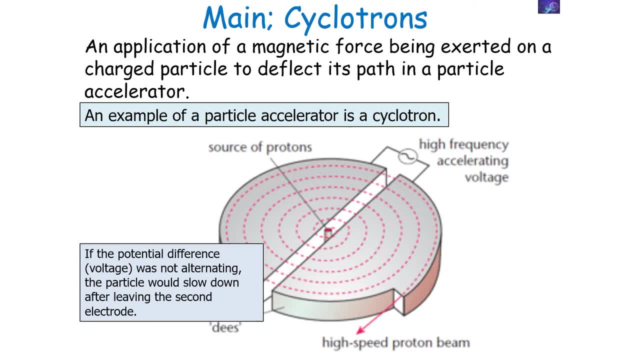 particle to slow down after leaving the second electrode because it would be going into a potential of like value, so it would repel. So the alternating voltage can change in a periodic fashion, as the time taken for the particle to move in the D semicircle doesn't depend on its speed. 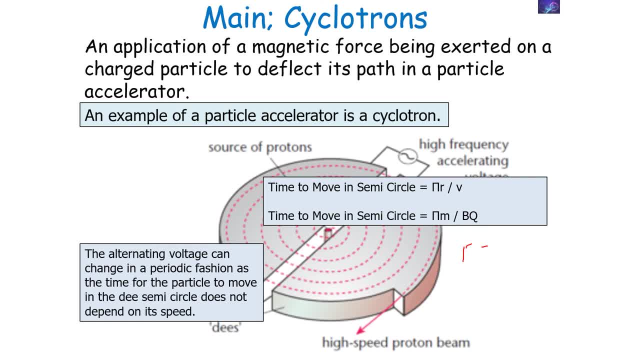 We know this because time to move in a circle is equal to distance over speed. so we know that the distance in a semicircle is pi R. Ok, So therefore we can say pi R over V. but we know that R is equal to mv over bq, so therefore, 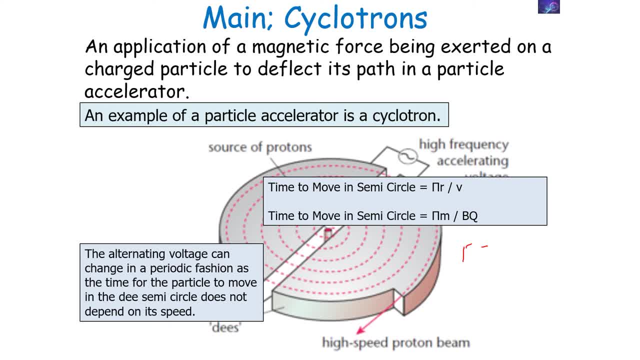 we can pop that into the equation and we can say that the time to move in a semicircle is pi m over bq, The second equation coming from the fact we've substituted R equals mv over bq into the first equation. Now the time equation we just looked at does not contain a velocity term showing that. 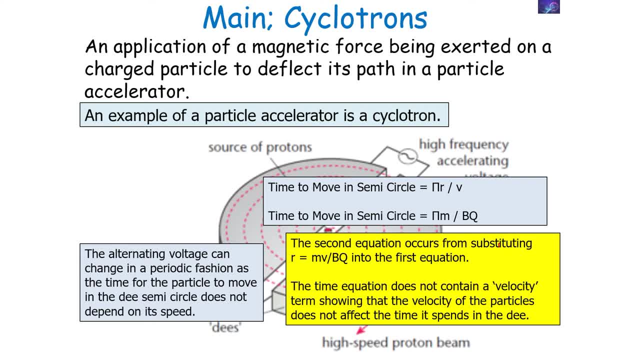 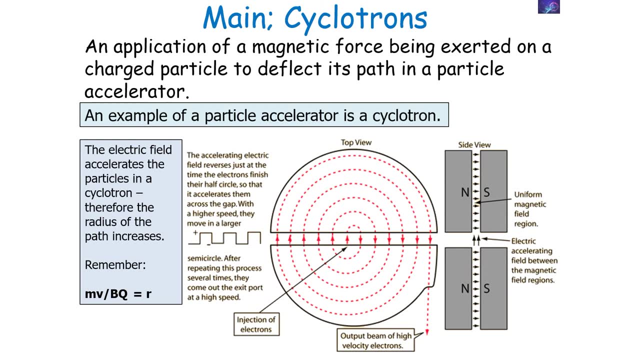 the velocity of the particles do not affect the time it spends in the D, because when the velocity increases the arc of the circular path increases to compensate, so it keeps the time taken to be constant in that semicircle. So just to clarify: the electrical field accelerates the particles in the cyclotron, so therefore, 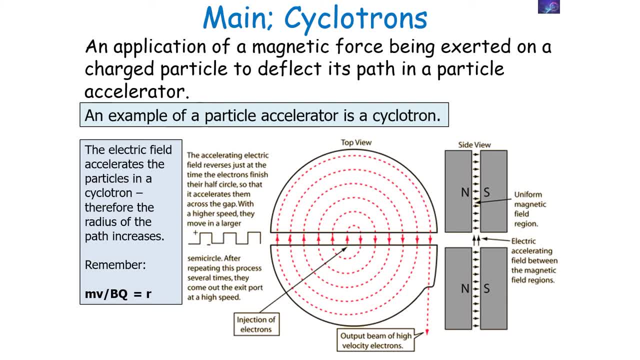 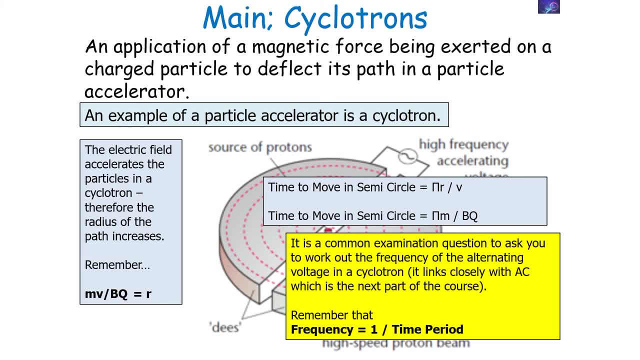 the radius of the path will increase, because R is equal to mv over bq. So what we can then do is we can look at working out the frequency of the alternating voltage in the cyclotron, which links closely to alternating current, because we know that frequency is. 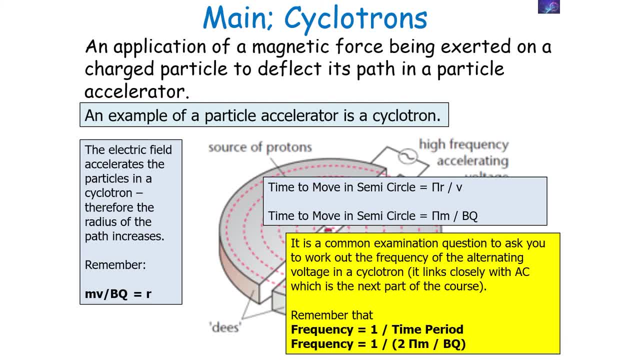 one over time period And we've worked out the time period previously to be 2 pi m over bq because, remember, the time period is the time it takes for one complete circle. so the time taken to move in a semicircle must be doubled. 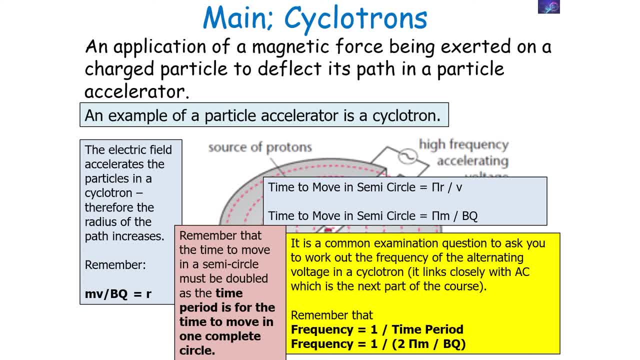 So time in a semicircle is pi m over bq, so the time period in total is 2 pi m over bq. So at this point you could then rearrange this equation and say bq over 2 pi m, and that gives us our frequency of how much we're going to alternate our potential difference. 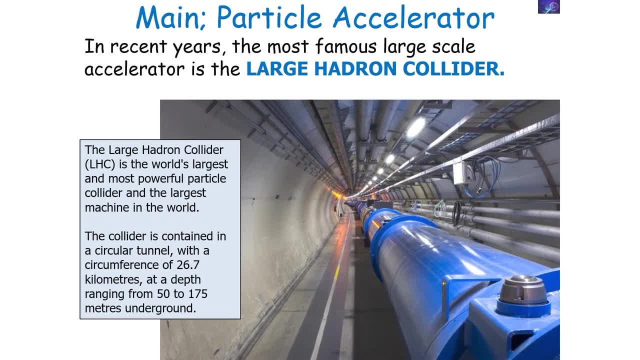 Now, this is real indeed. So the following would be the paradigm here, and I just want you to remember that, the moment we get to the last step, and remember the 1 pi m over bq, we're going to be alternating current over the cycle. 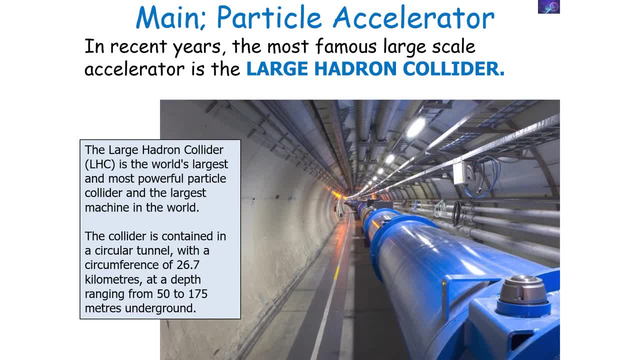 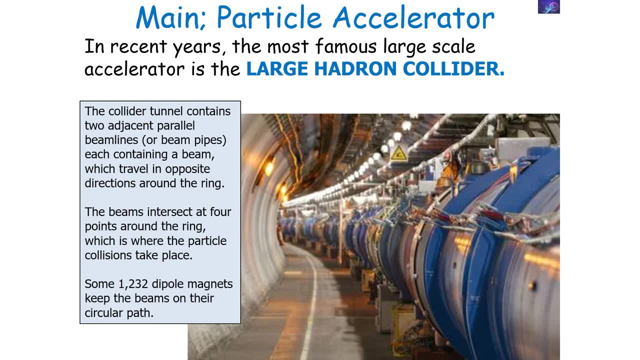 So if you want to see how we can see how the cycle is going to be, please go back to the situation and remember that you can't do that with a single cycle. You can't do it as a single cycle. So you're going to be alternating current over current over current at the end of the cycle. 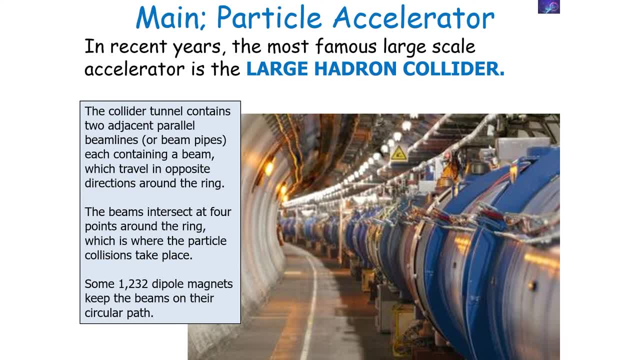 So the minimum that's going to happen is that the cycle is going to be 2 pi m over bq. You can look at the cooking of the air, you can look at the temperature of the air and place and we've got about 1,200 dipole magnets to keep the beams on their 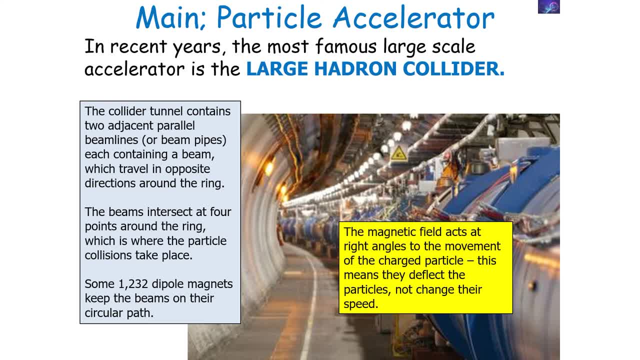 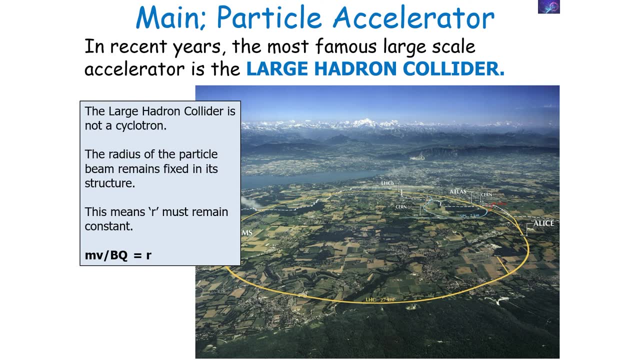 circular path. Now the magnetic fields act right angles or perpendicular to the movement of the charged particles, which means they accelerate by deflection, not by changing speed. Now the Large Hadron Collider is not a cyclotron. The radius of the particle beam remains fixed in its structure, So this means R must. 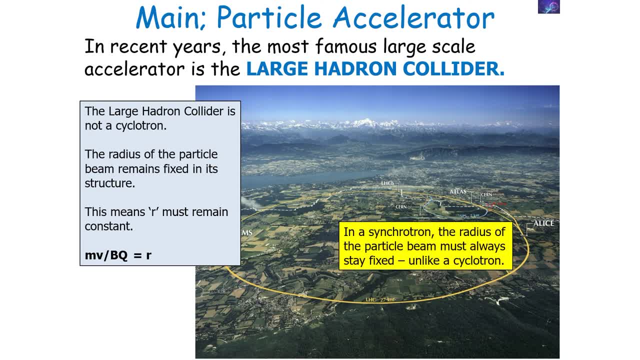 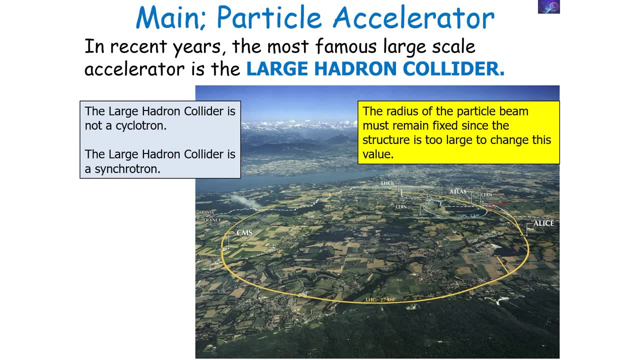 remain constant in the equation. This is what we call a synchrotron. So in a synchrotron the radius of the particle beam must always stay fixed, unlike a cyclotron. Now. the radius of the particle beam must remain fixed since the 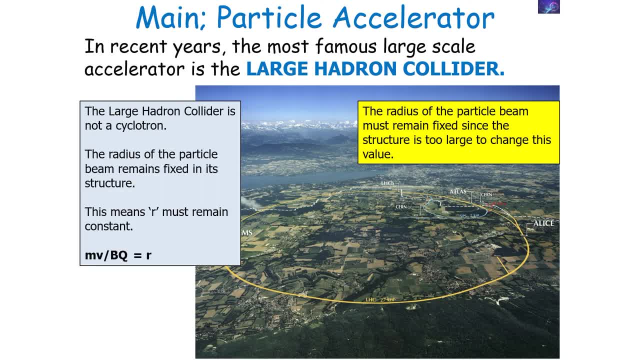 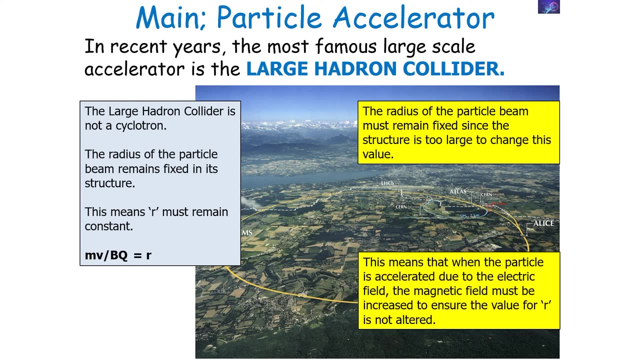 structure is too large to change this value, So the radius of the particle beam must remain fixed, otherwise the particle beam would hit the side of the actual collider. So, as a result, we've got to look at the actual value of R that we've got. So this means that when the particle is accelerated due to the electrical 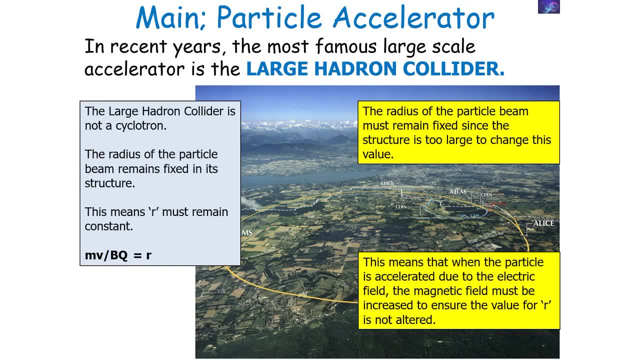 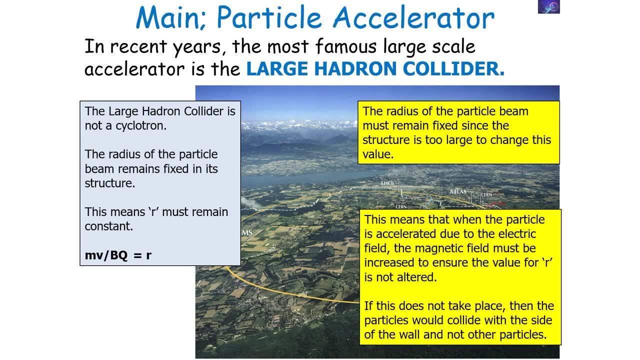 field. the magnetic field, must also be increased to ensure the value for R is not altered, because the increased B value in the equation cancels out the increased V value. Now, if this doesn't take place and the particle will collide with the side of the wall and not the other particles, 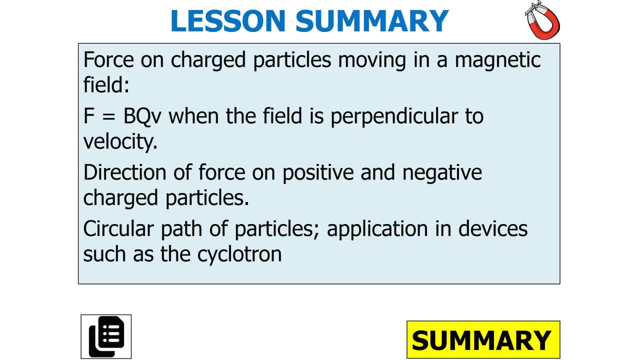 So let's summarise what we've learned in today's lesson. Forces on charged particles moving in a magnetic field are given by the equation F equals BQV. when the field is perpendicular to the velocity, The direction of the force on positive and negative charged particles can be calculated and we understand the. 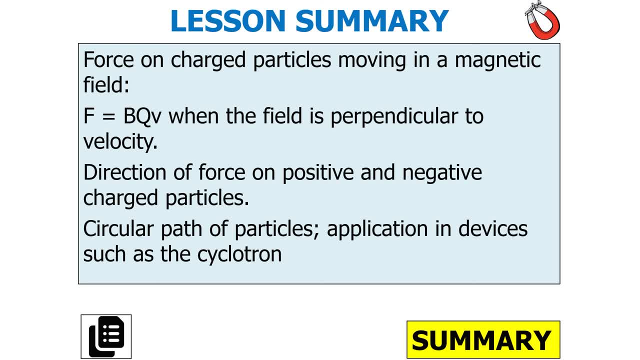 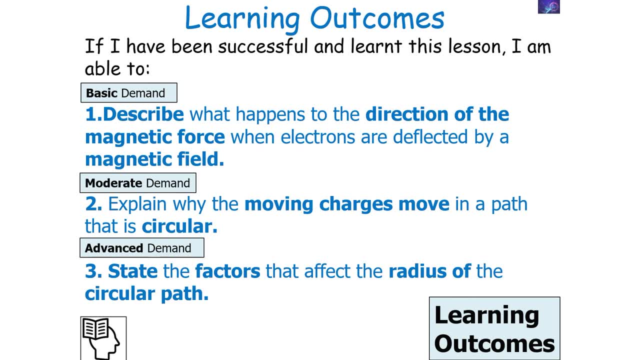 circular paths of positive and negative charged particles are calculated by the equation. So I hope you've been successful and learnt in today's lesson, where we can describe what happens to the direction of the magnetic force when electrons are directed by a magnetic field. We can explain why the moving charged particles move in a path that.